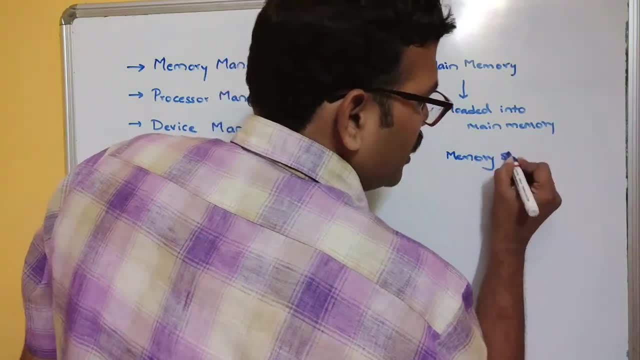 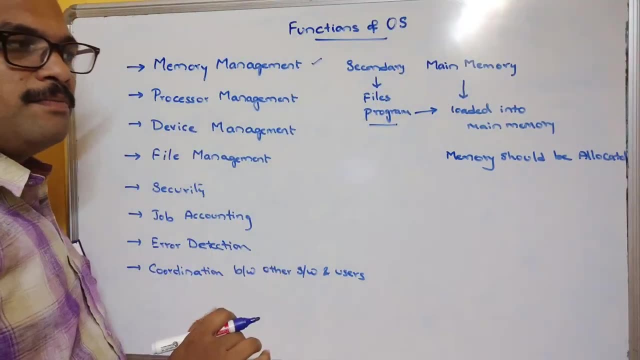 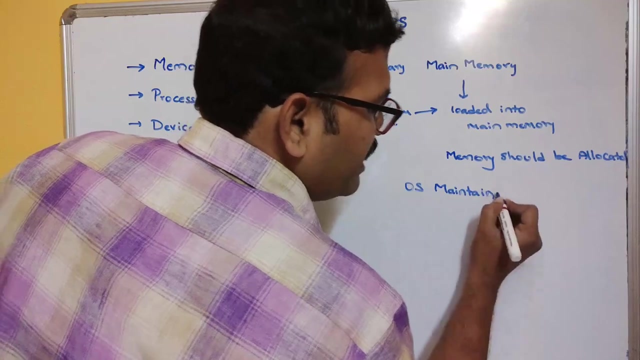 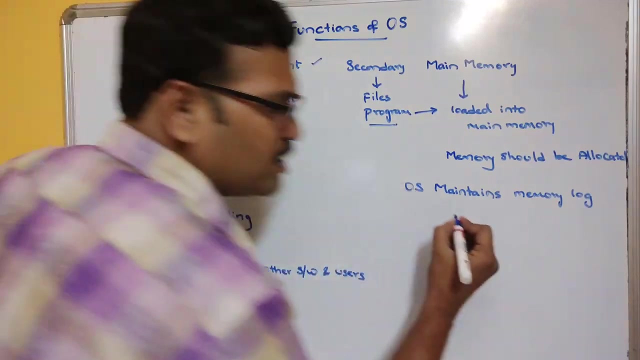 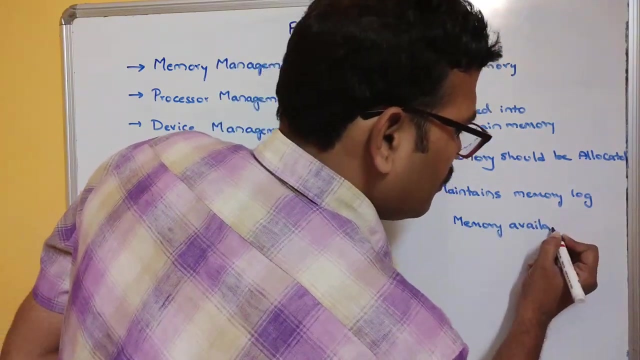 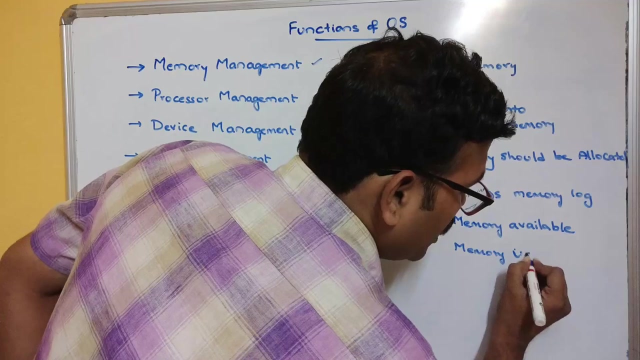 memory should allocated, should be allocated, right. so operating system will maintain this memory log. okay, so os maintains a memory log. so memory log means it keeps on. keeps on tracking about this memory. that means which memory is available, which memory is available, which memory is available and which memory is used. so this is very important because so whenever the operating system 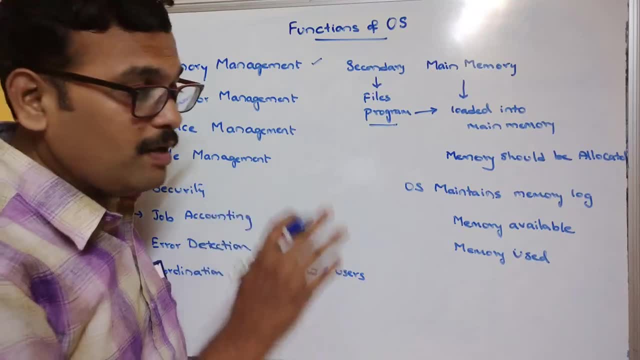 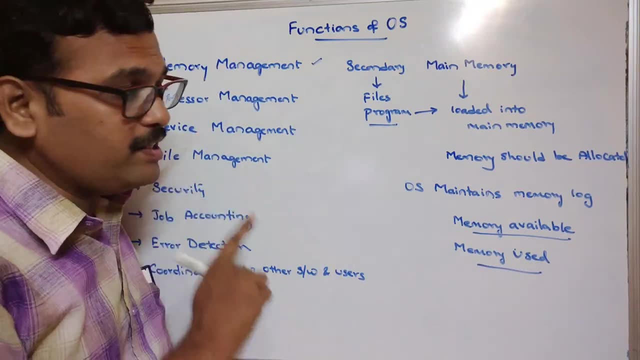 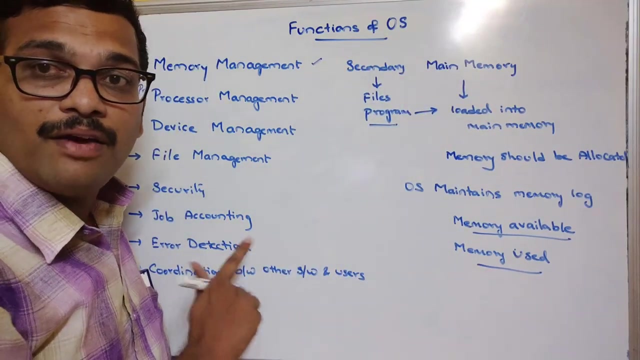 wants to allocate a memory for a process or a program, first it have to know which memory is available, which memory is already allocated. so the operating system will allocate the memory whenever the program is loaded into the main memory for the execution, and whenever it requires a memory, it will allocate the memory for the execution. so this is very important because 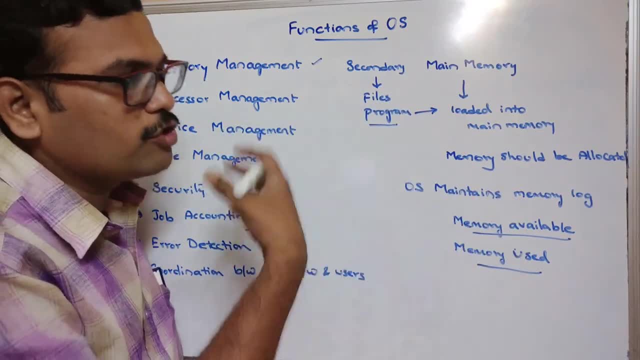 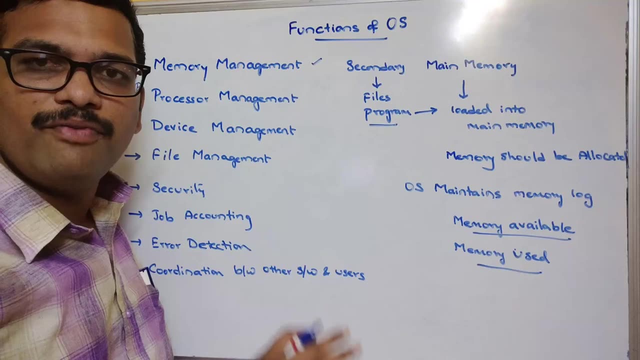 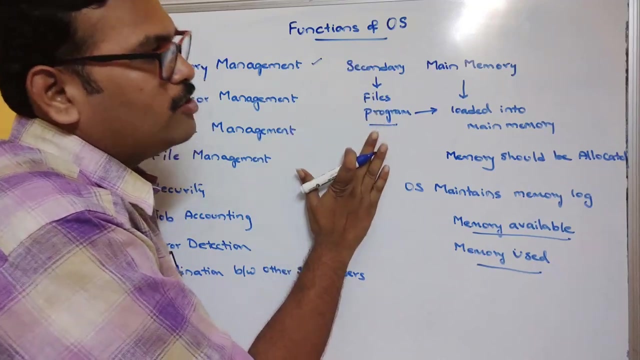 any io operations or whenever the process execution is completed or the memory will be deallocated by the operating system itself. so allocation of memory and the deallocation of memory will be done by the operating system, right? so hope you understood. so the programs or processes should be executed by loading it into the main memory. so some sort of memory should be. 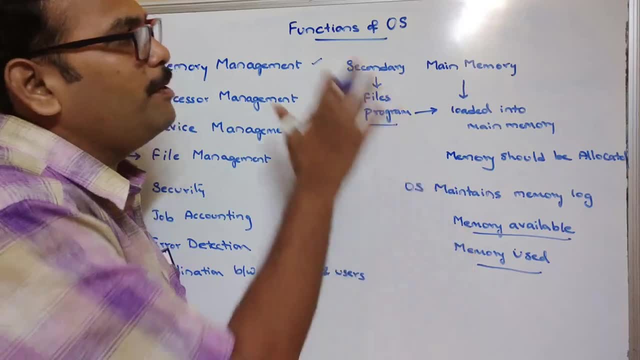 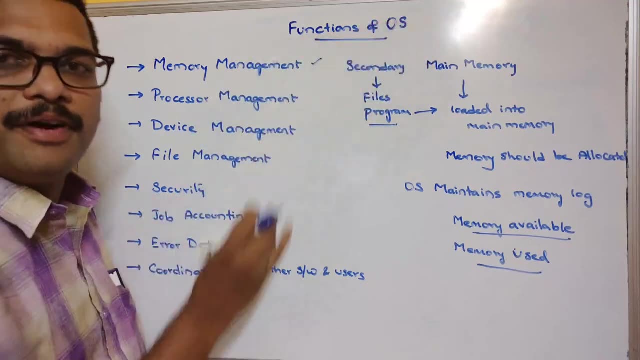 allocated for that particular process and that particular thing will be maintained by the operating system. then that process we call it as a memory log. so this is very important because memory management, so this will be done by the operating system. this is one functionality done by the operating system. so allocation of memory to the 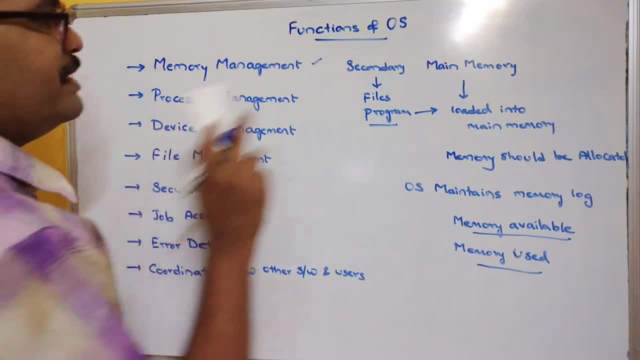 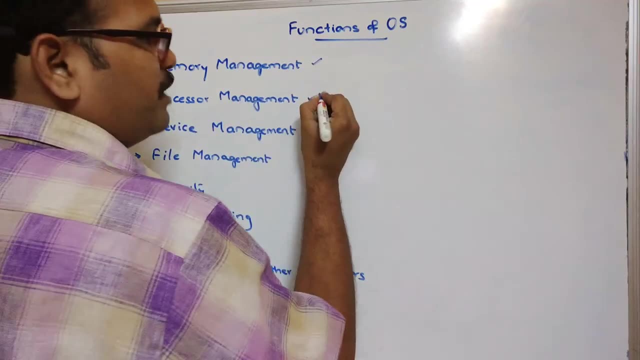 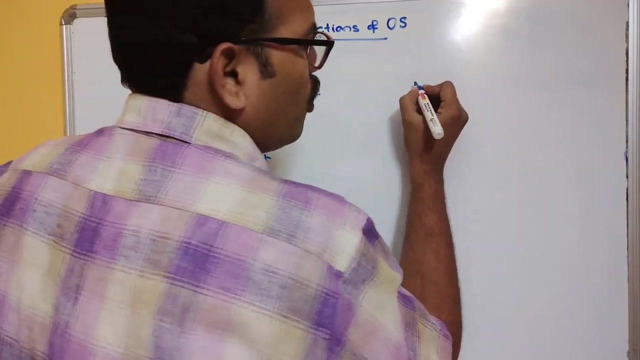 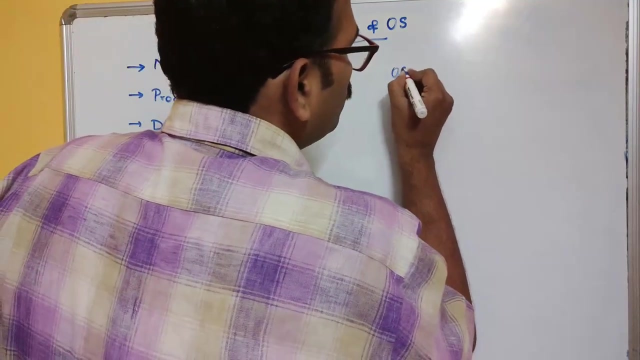 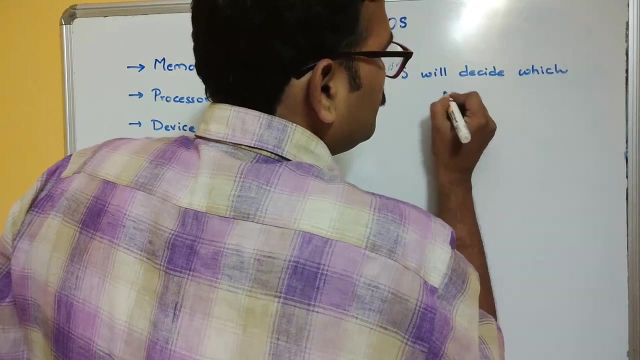 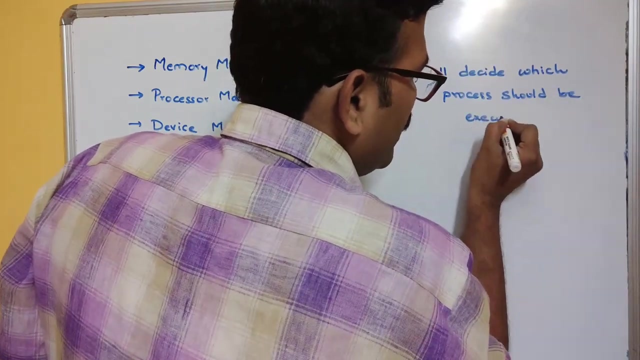 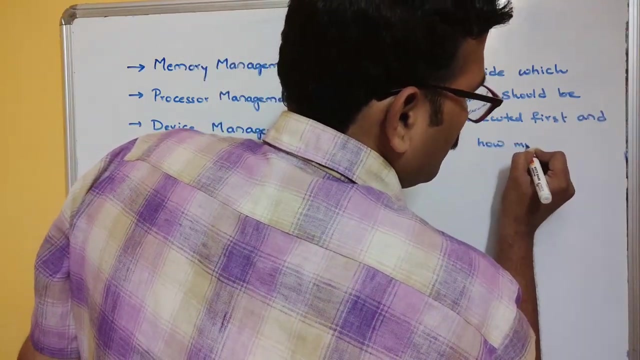 program to be get executed. then next one, processor management. processor management. so here the processor management means we will be having a lot of processors available in the queue to be get executed. so operating system will decide. so OS will decide which process should be executed first, executed first and how much time it. 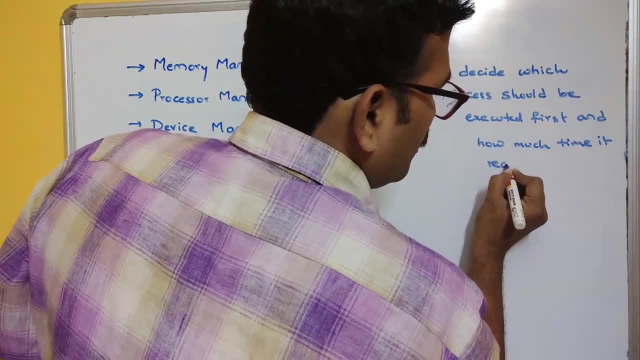 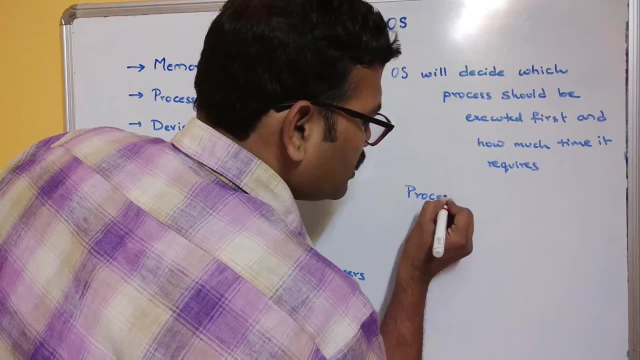 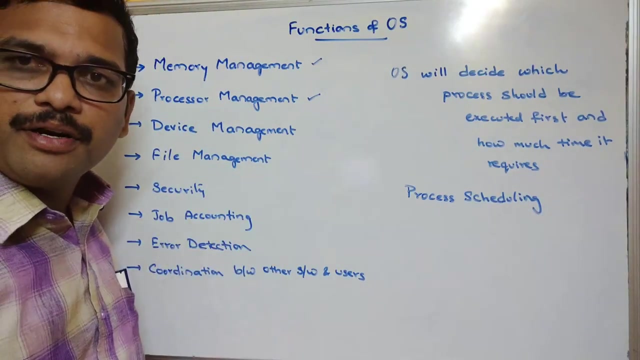 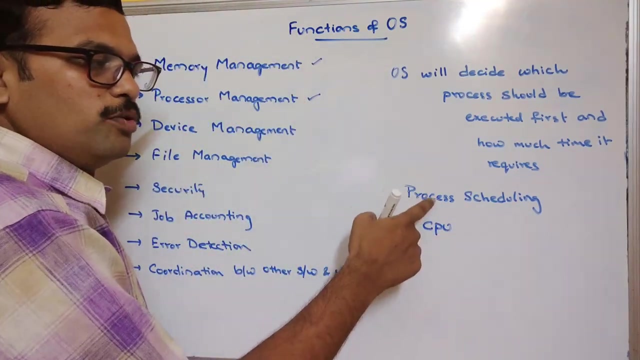 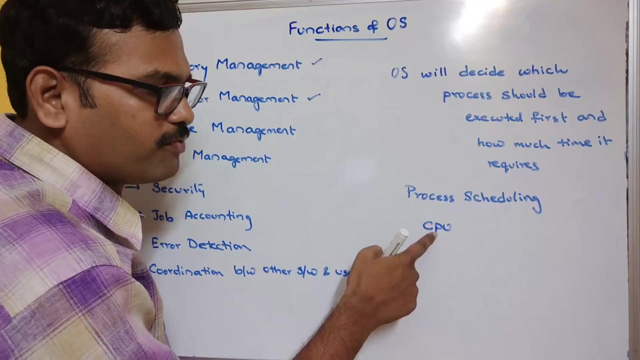 requires, it requires. so this will be done by this process and this process we call it as a process scheduling, process. scheduling, that means which process should be get executed right. so execution of the process will be done by the CPU. so the process should be given to the CPU. so the OS we add will do the access of CPU. 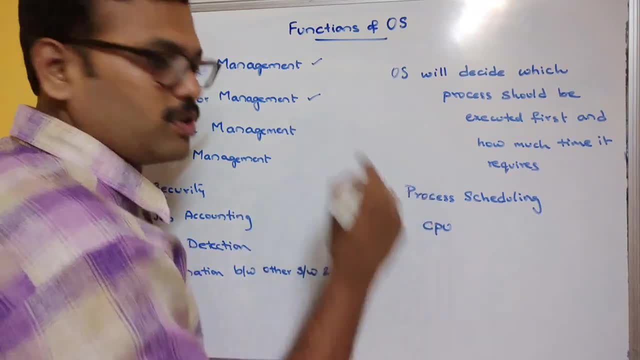 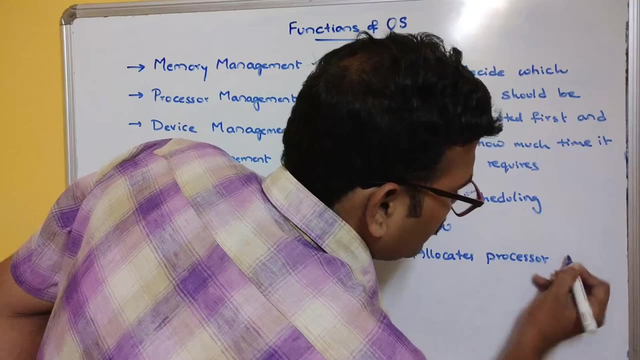 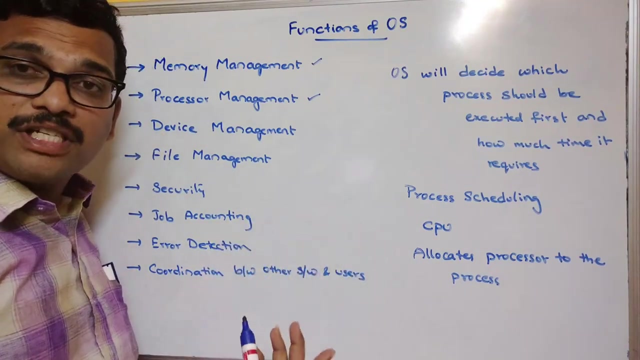 to the process. okay, allocates the processor to the process. so allocates processor to the process. so this sort of allocation, so after completion of the process- that means whether it can be a terminated or it may be waiting for the Ivo operations- then it will be deallocating the 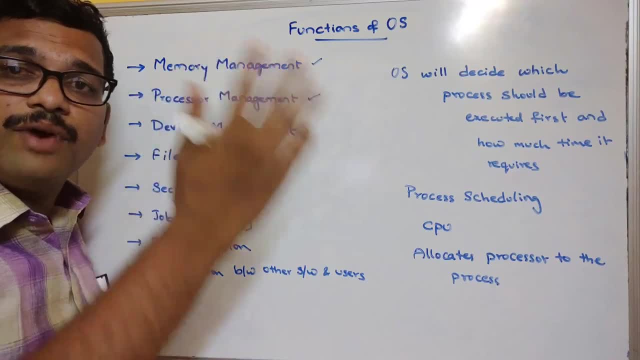 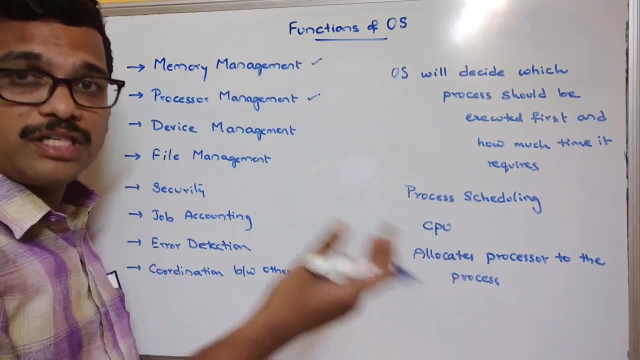 processor because so whenever it works with the Ivo, devices automatically instead of making the CPU in idle. so CPU will be allocated to the other process, so that we have seen in the multi-programmed operating system, so that we call it as a multi-programmed right. so 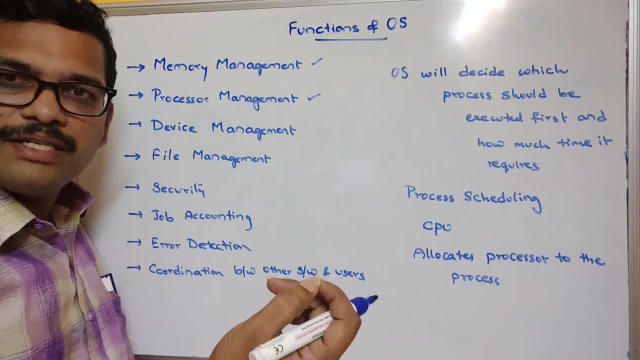 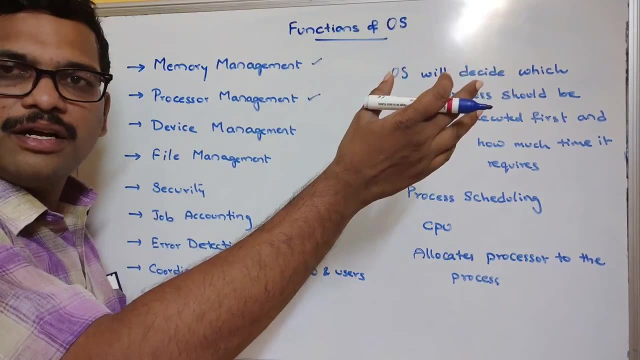 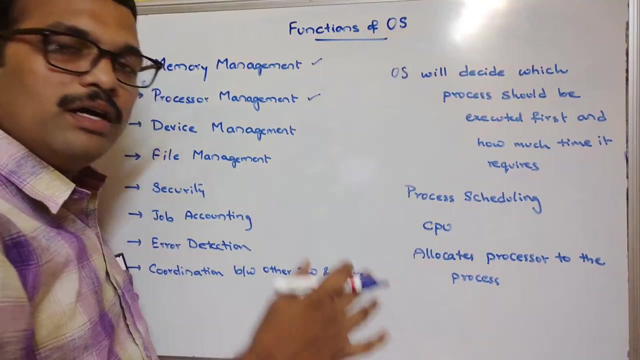 whenever the process requires for the Ivo devices. so automatically the CPU, instead of keeping the CPU idle state, the CPU will be allocated to the other process, right. so the allocation of processor to the process will be done by the operating system also. the deallocation will also be done by the CPU. 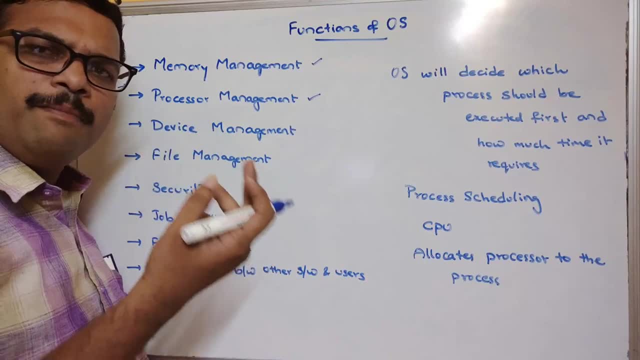 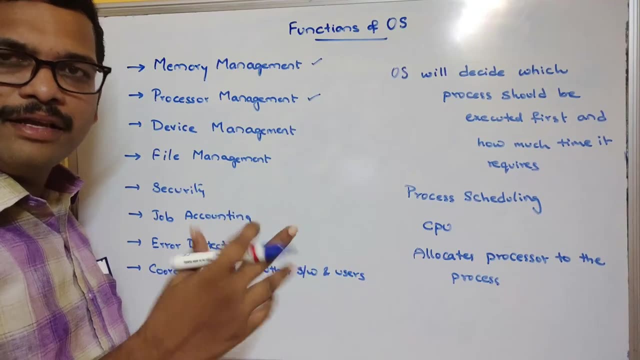 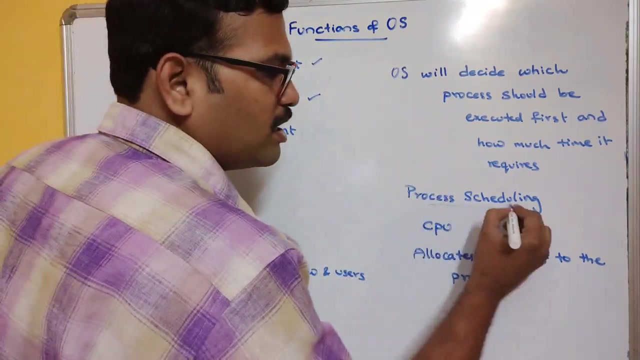 So the deallocation means it may be the processor completes its execution or it may be waiting for the Ivo operations. so anything in any case, the deallocation of processor will also be done by the operating system, and this process we call it as a process scheduling process. 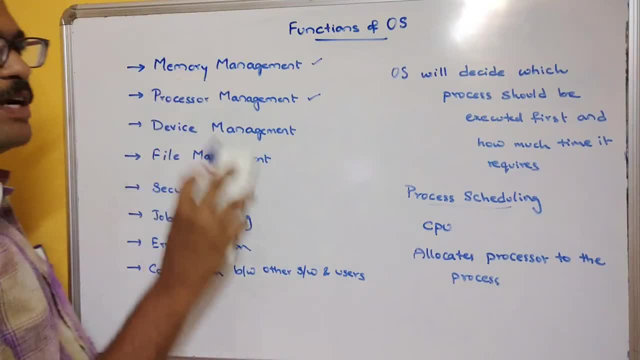 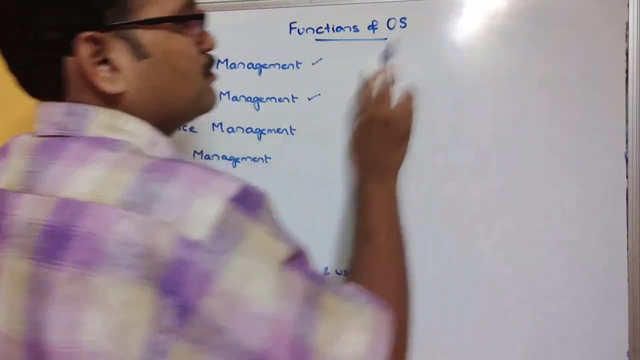 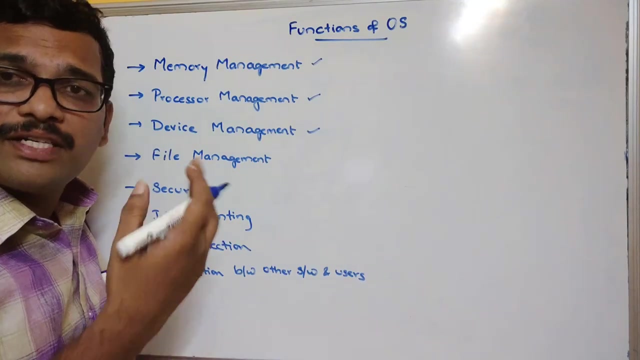 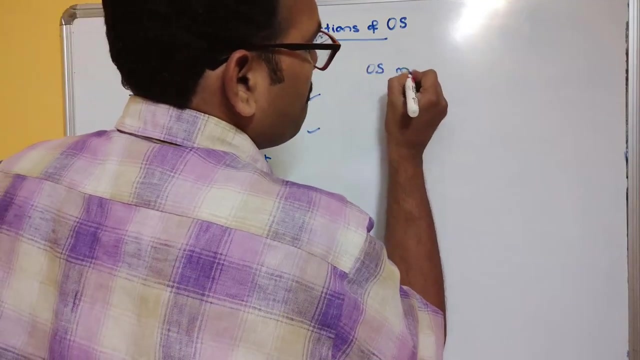 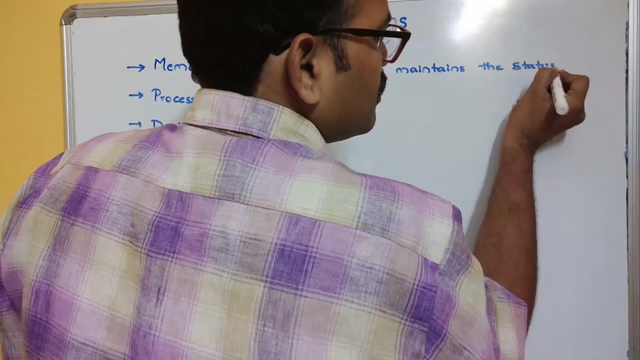 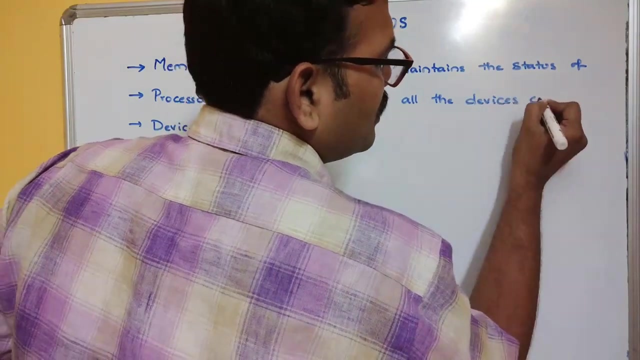 scheduling right, so hope you understood this. one: processor management, so allocation of a processor to a process. next one: Device management, so during the execution of a program, so it may require some Ivo operations, so in that time. so all the devices, so OS maintains the status of all the devices, all the devices. 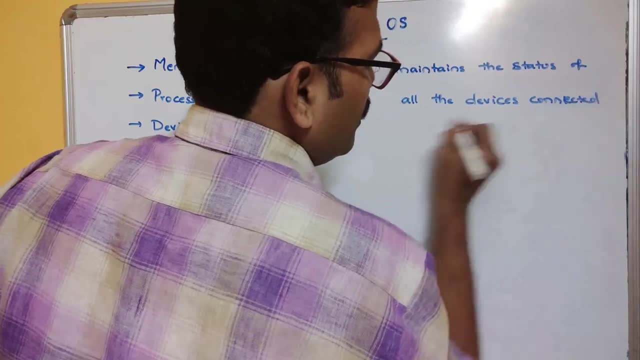 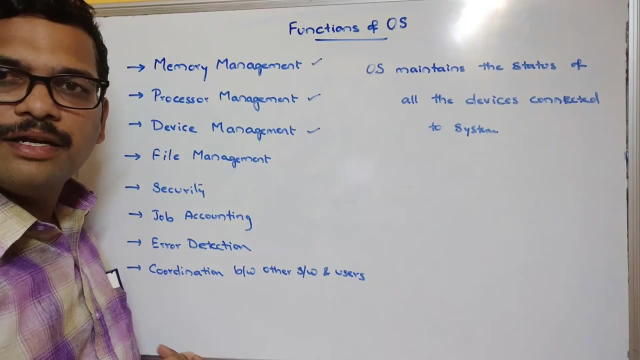 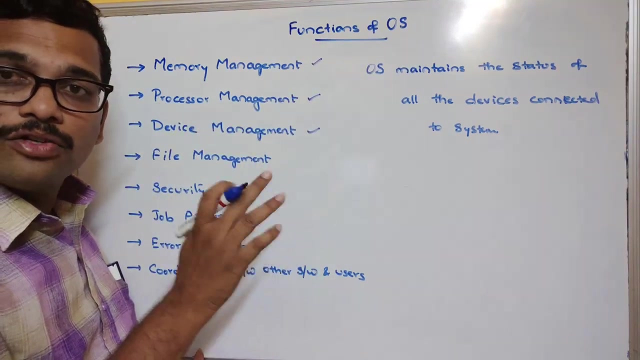 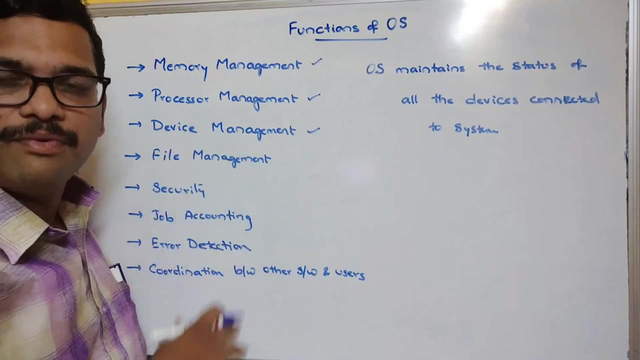 connected to the system. Connected to the system, so whenever the process wants the Ivo operations, so this particular operating system will allocate the device to the operating system and also it will keep track on how long it requires the device, how long it maintains the device right. so everything. 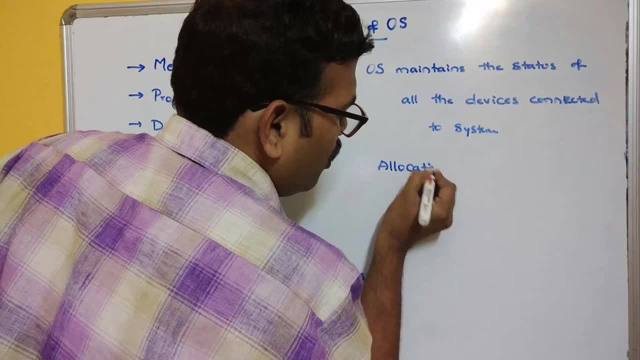 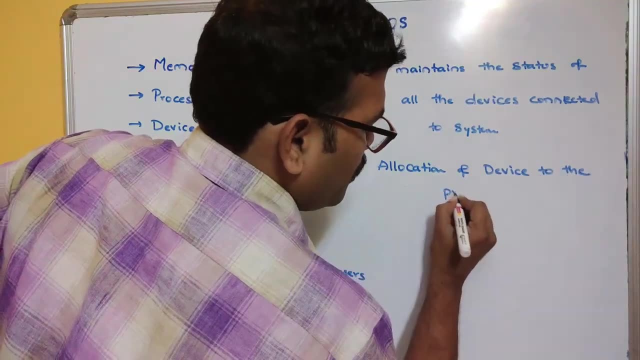 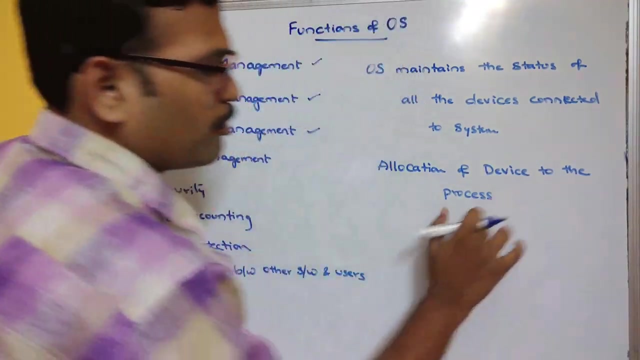 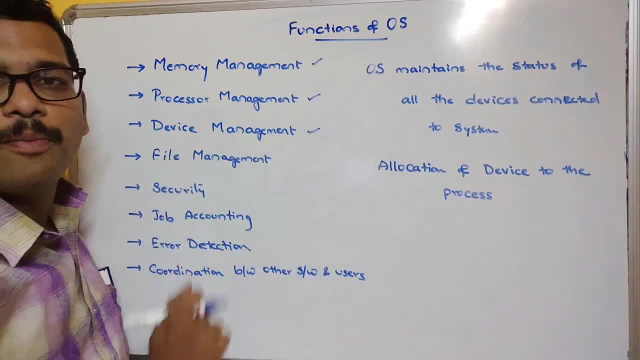 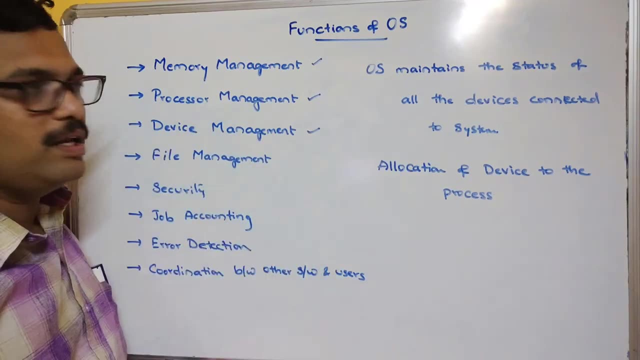 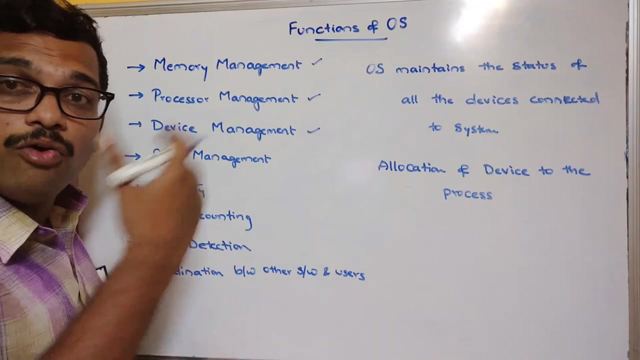 automatically. the deallocation of the device will also be done by the operating system itself. So whenever the during the program execution, whenever it requires Ivo devices, Ivo operations, automatically, the operating system will allocate the device. so it should maintain the status of all the devices connected to the system and how long the device is using by the process, everything. 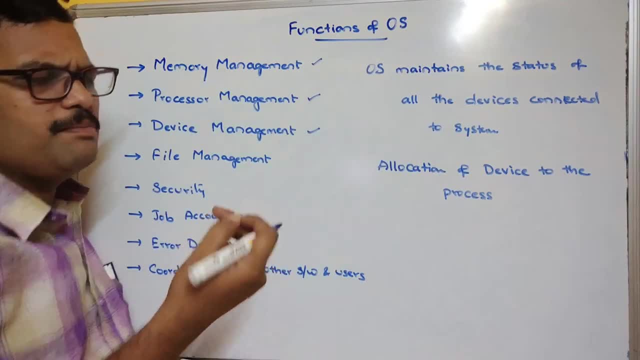 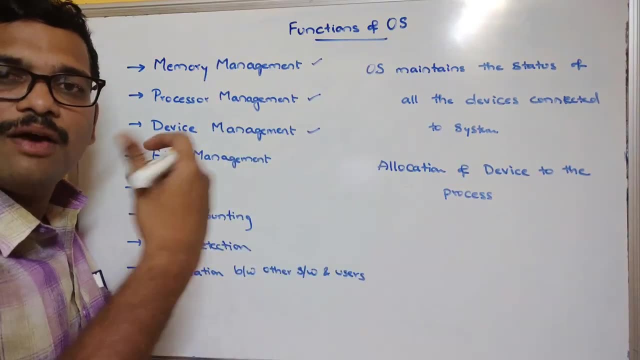 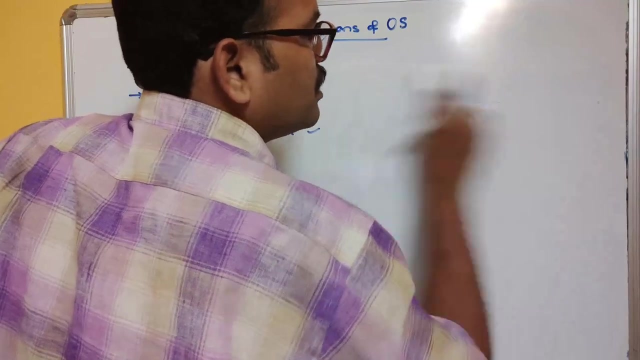 everything related to the device, so we can simply call it as a device log. device log will also be maintained by the operating system in order to allocate and deallocate the devices to the process whenever it is required. right, so this is called the device management and the next one the next. 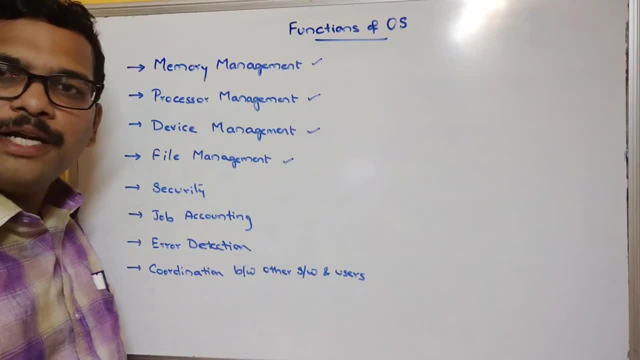 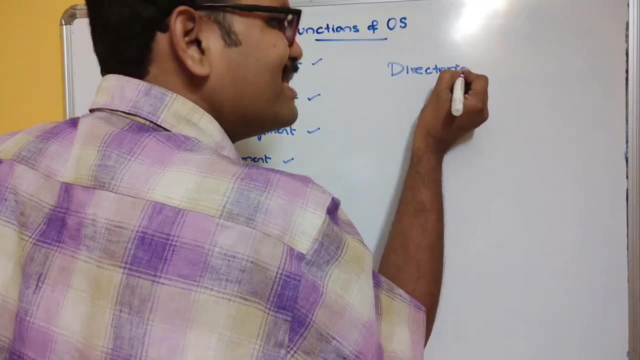 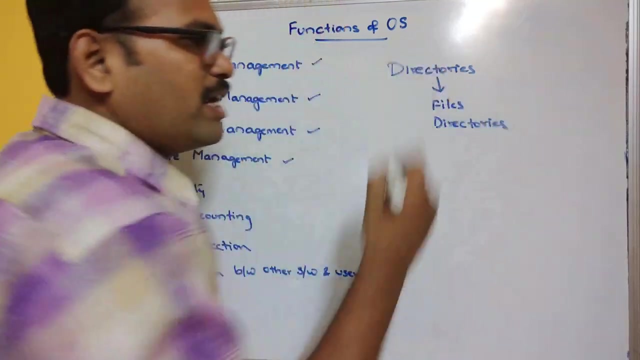 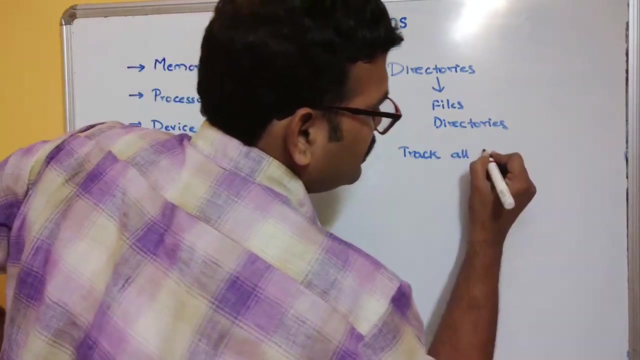 one file management. coming to the file management, so actually the programs will be stored in directories. in directories and inside the directories we can have files and directories, also right directories. so we need to keep track on each and every file. so os will track all the file status. 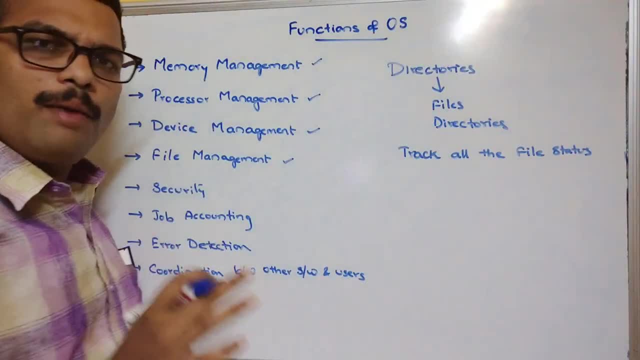 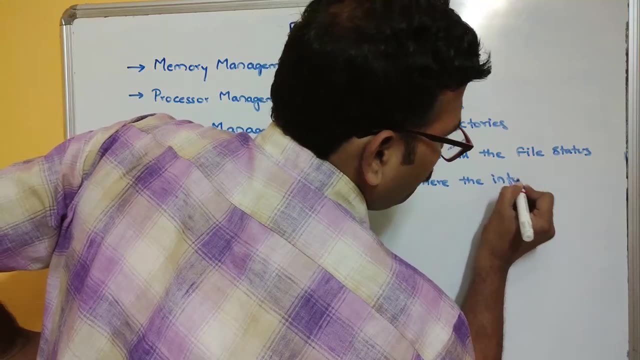 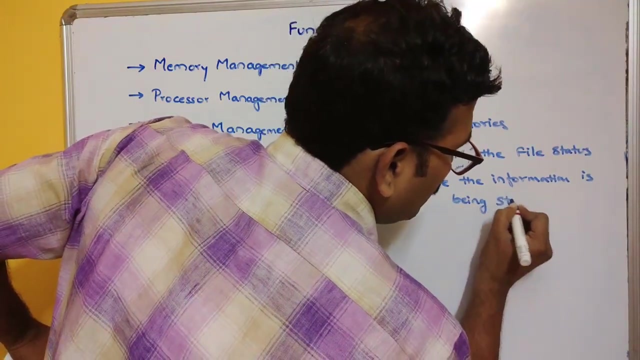 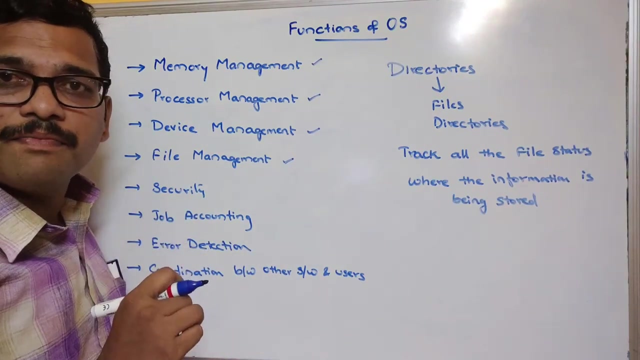 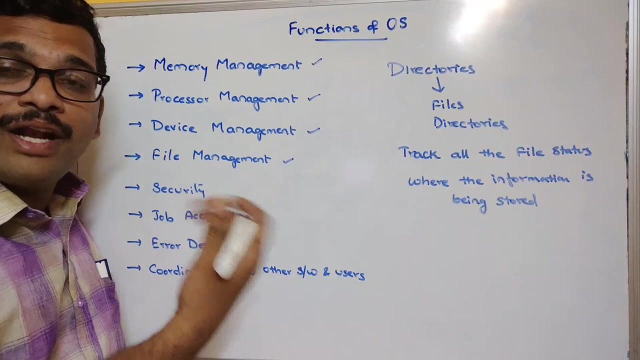 right, it will know about the information where, actually, where the information is stored. information is being stored, so this will be done by the operating system itself. so where the information is being stored, right so the file system, the file system, the data is the information will be stored in directories or files and where it was located, right so whenever it is required, 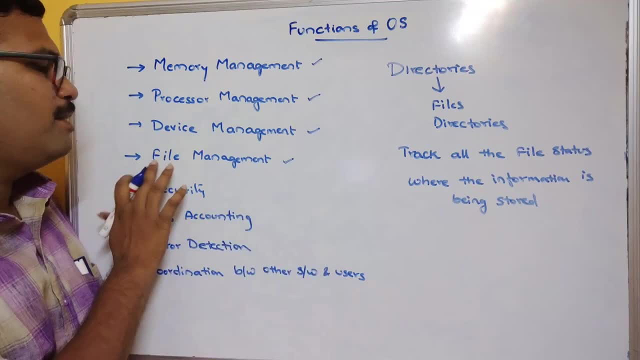 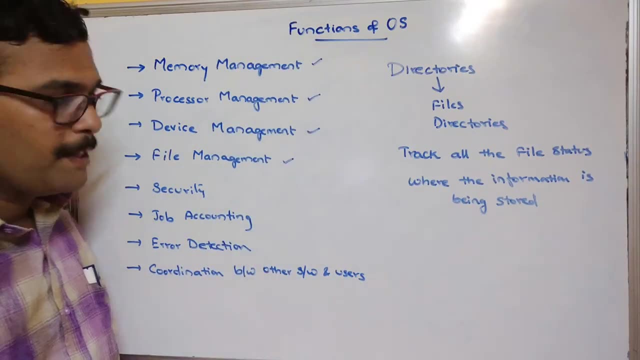 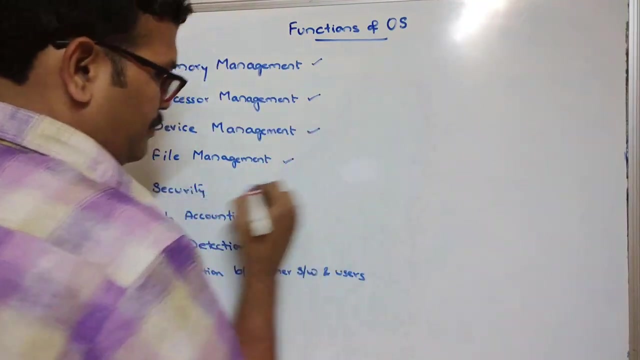 the data from the particular file so that complete log will be maintained by the file management and that process. we call it the file management. it is maintained by the operating system, it will be done by the operating system and next one is a security security. so os provides the security os provides. 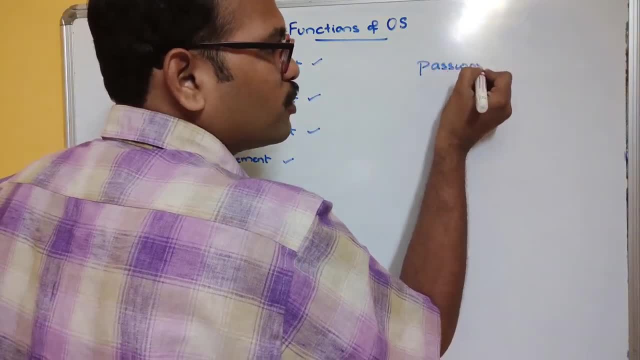 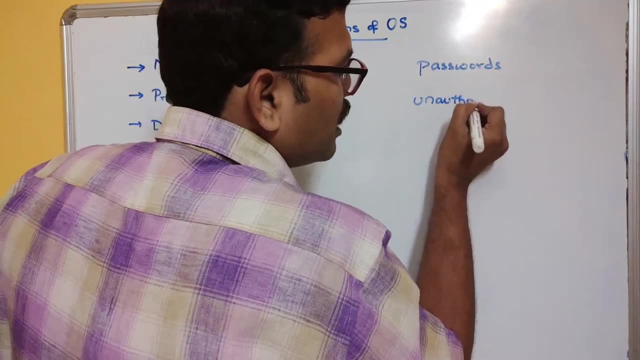 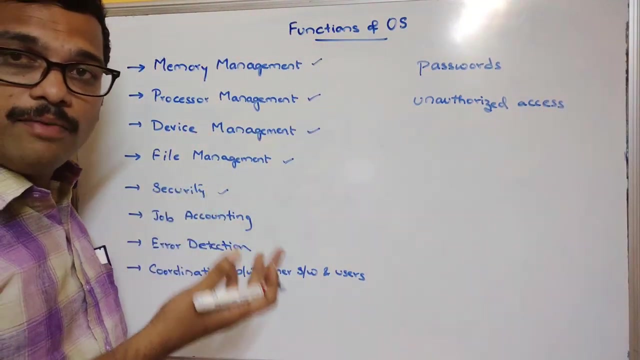 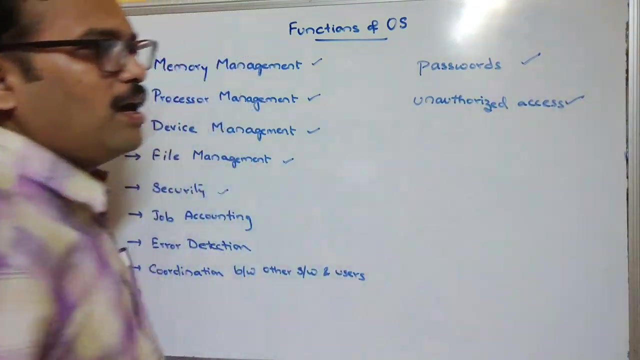 the passwords for different users so that it can be the data can be protected from the unauthorized access- unauthorized access, unauthorized access right. and also it maintains a log. okay, it maintains a log of all the users, right? so by using these passwords and passwords, the security will be provided for. 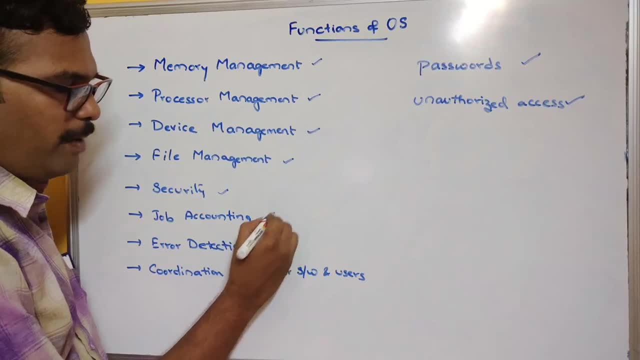 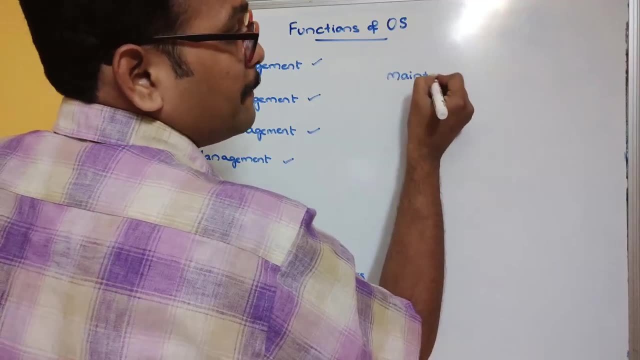 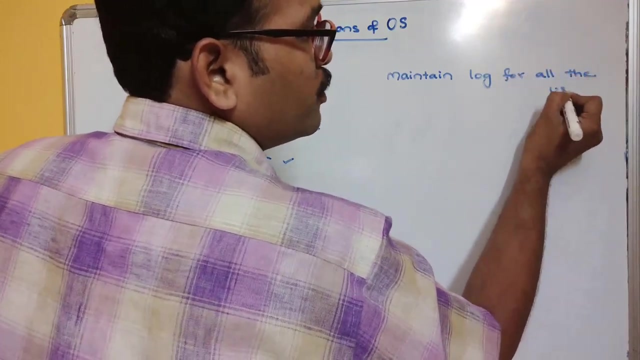 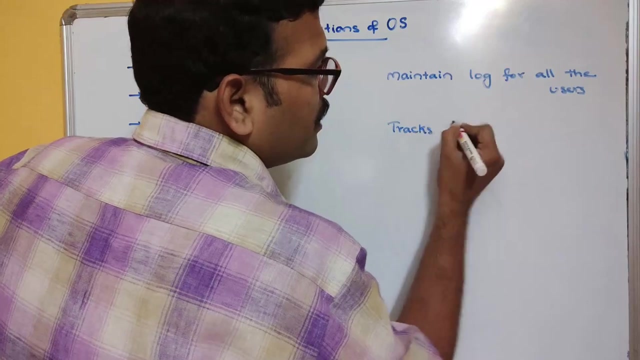 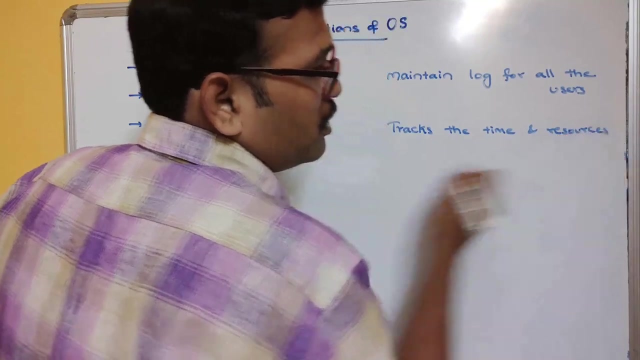 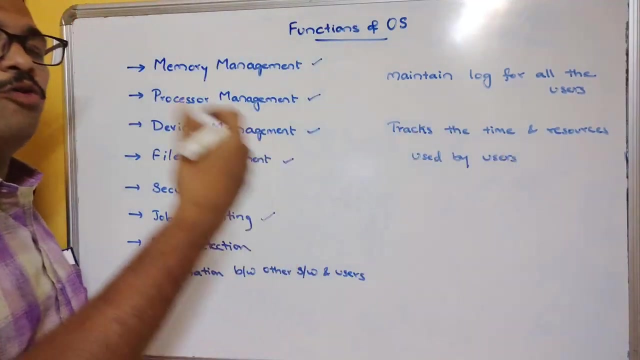 the data. and coming to the job accounting, job accounting and os will maintain a log for all the users, all the users. so here the log means it will keep track. it will track the time and resources, the time and resources used by the users, how much time and how how much. how many resources are being? 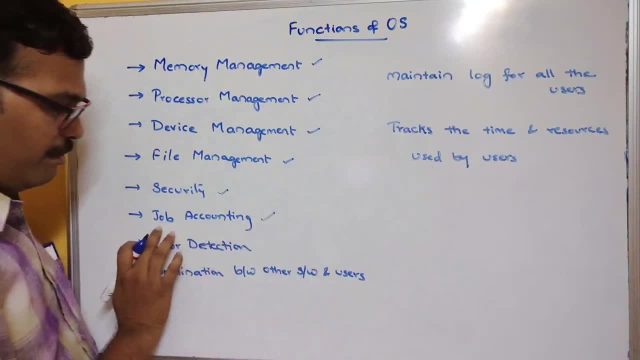 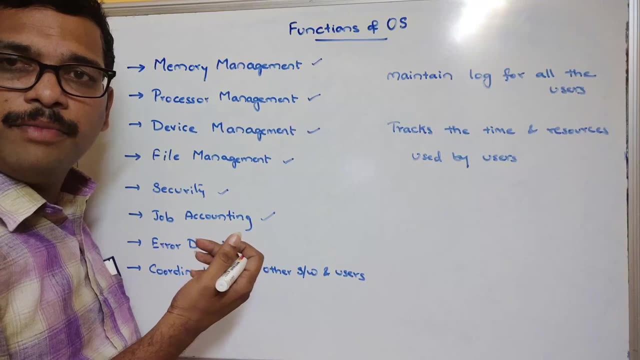 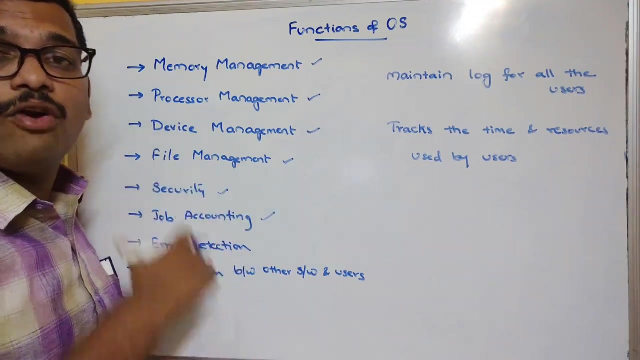 used by the users. so this log will be maintained by the operating system and that is the job accounting right. so we'll be having a more number of users by log. by giving a login, it will maintain a more number of users so that the data which was created by one user cannot be accessed by another. 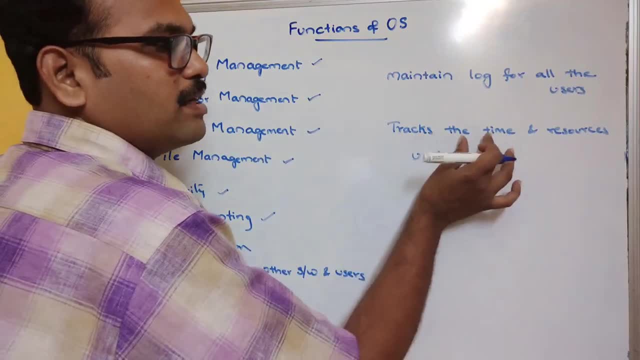 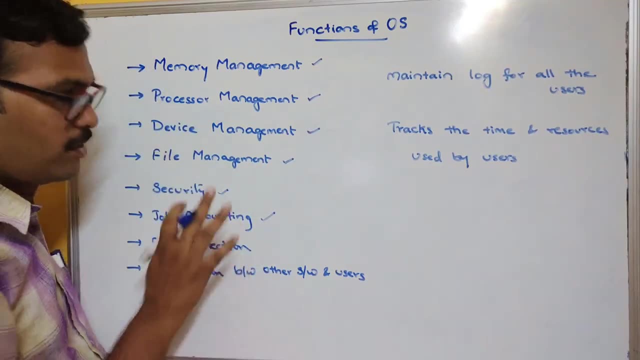 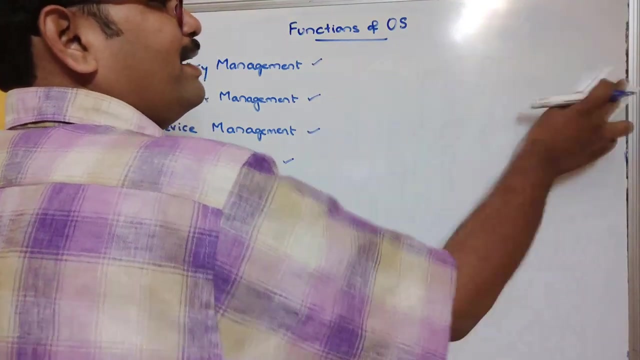 so for that it will keep tracks the time and resources used by the users, so how much time they are using the resources and everything, everything related to the user will be maintained in this job accounting. and the next one is error detection. error detection, so this error detection means 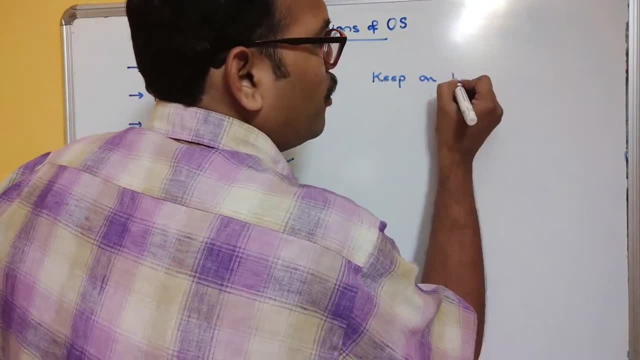 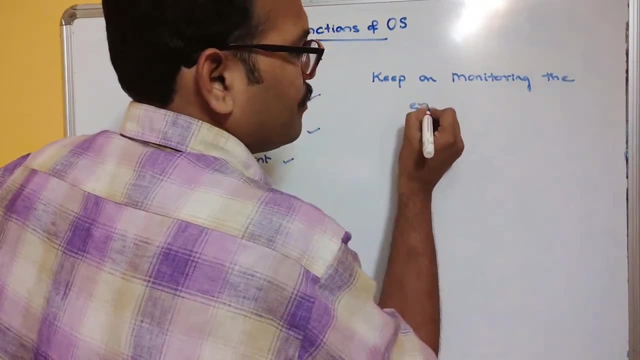 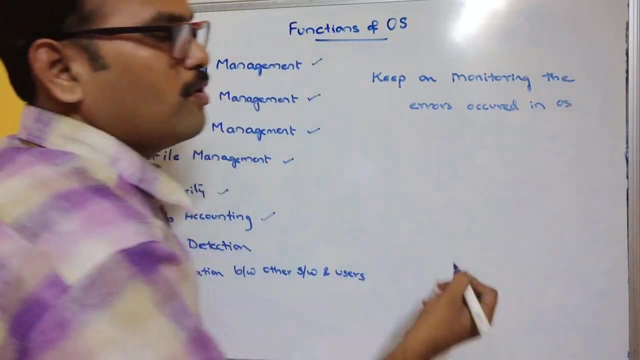 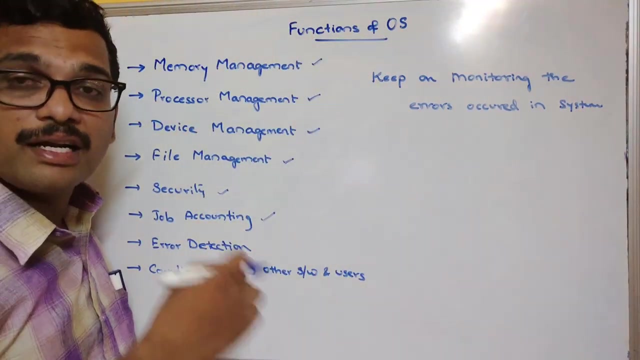 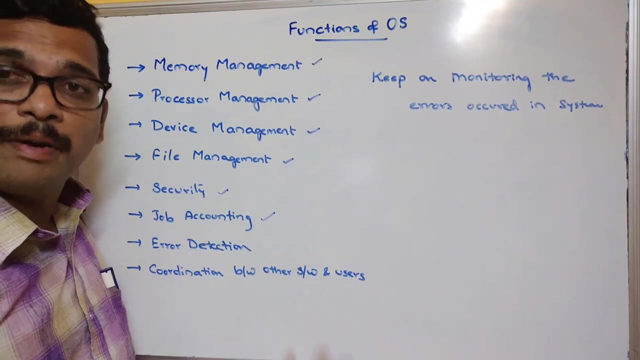 the os keep on monitoring the errors occurred in os or in hardware or anything okay, in the system. simply we can write it as system. that can be either program- the errors may be occurred in the program- or in the hardware, like ivo, this, ivo devices, or as a processor, so memory, whatever it may be. so all the errors will be keep on. 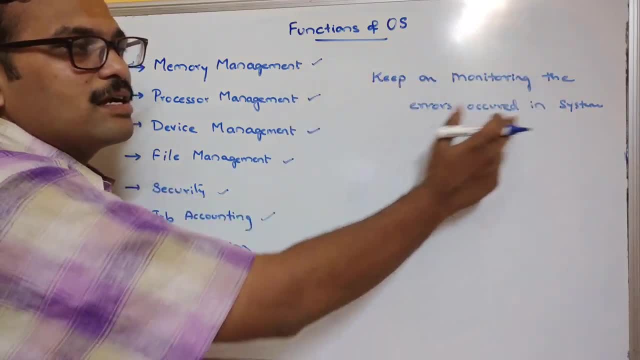 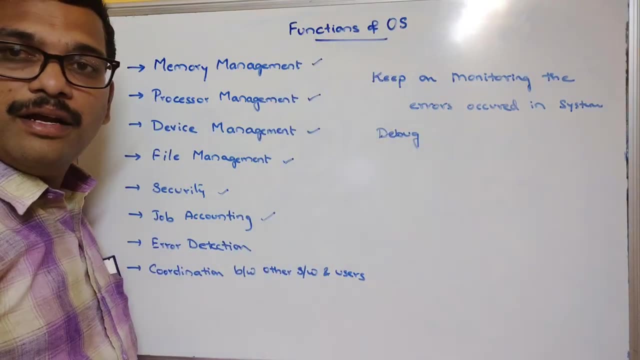 monitoring, i mean the operating system will be keep on monitoring the errors occurred in the system so that, whenever it is required, the db debugging process will also be done by the system, the OS right, in order to avoid the malfunctioning of a computer. okay, to avoid the malfunctioning. 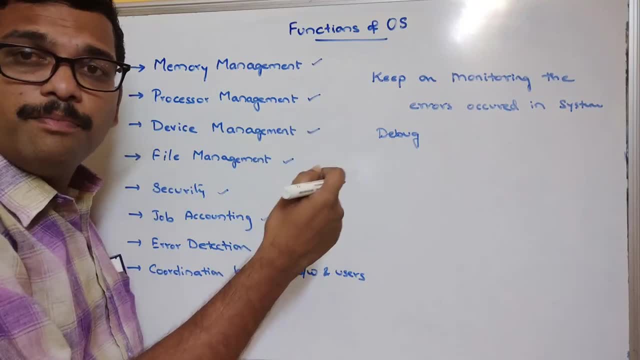 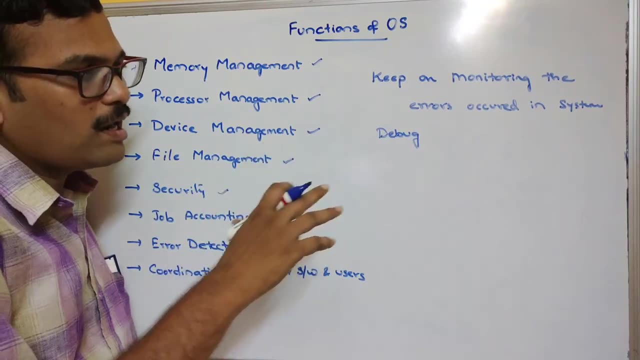 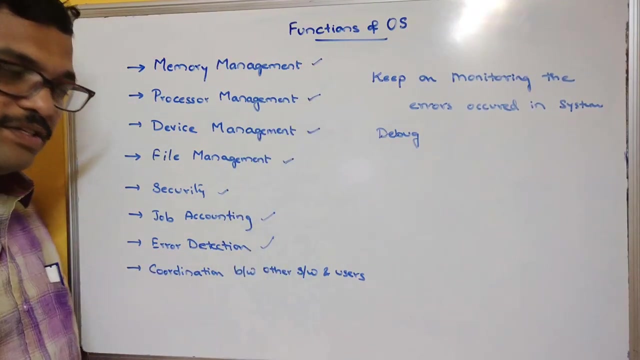 so sometimes it will debug and sometimes it will be sending the report of these errors to the user so that the users can take a certain action towards that particular error and to rectify the errors. so that will be done by the operating system and it is called the error detection. 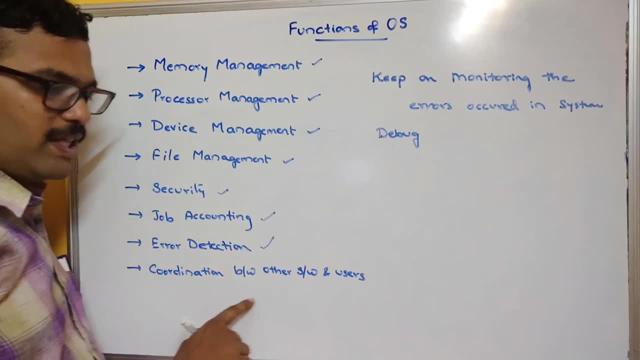 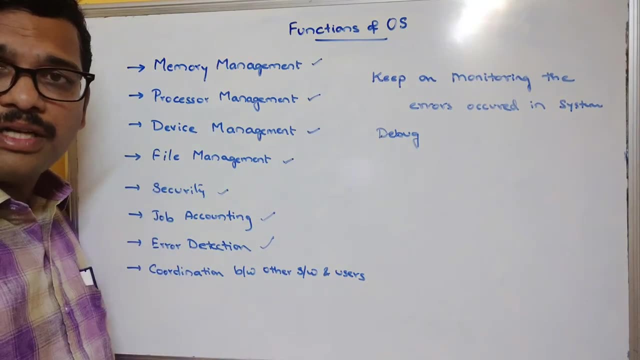 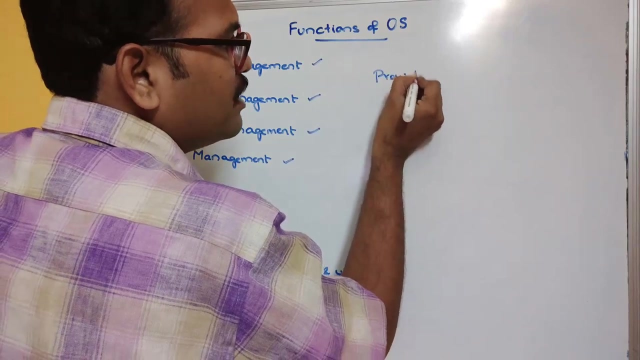 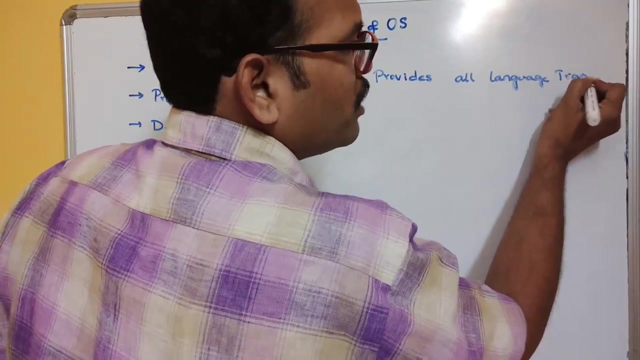 error detection. and the last one, the coordination between the other softwares and the users. so the system will be used with the- I mean by the different users and different softwares, so the OS will provide it. the OS provides all the language translators, language translators, so we know that language translators, so this language translators are. 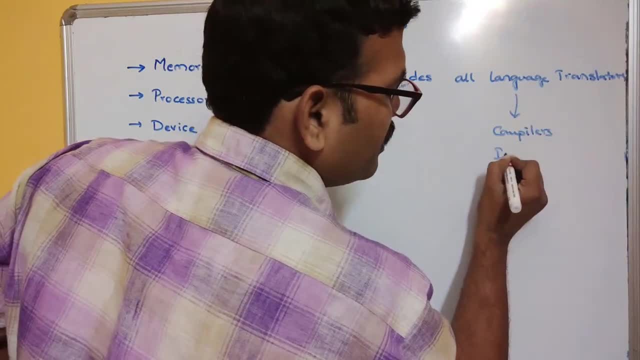 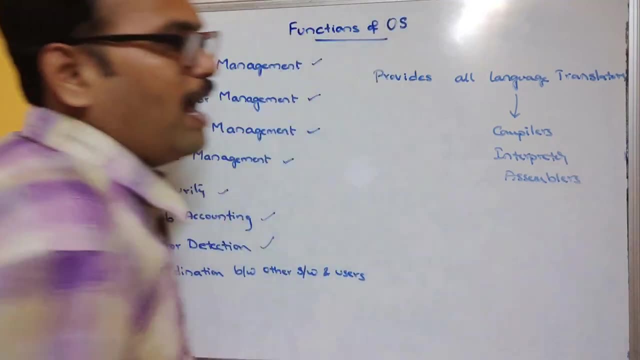 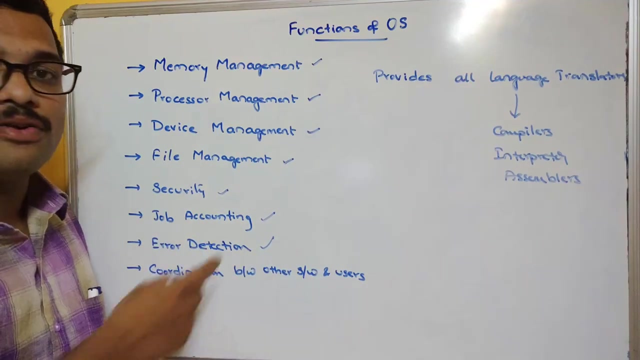 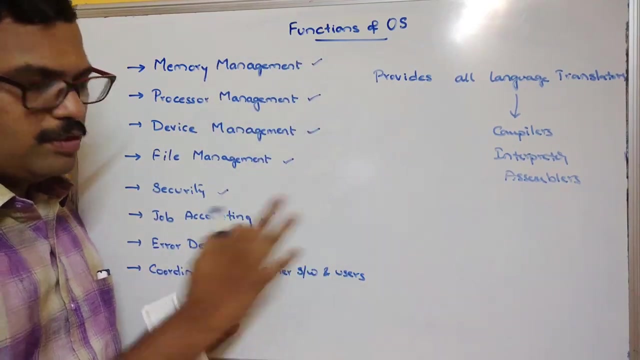 the compilers, the No interpreters, assemblers, so all these will comes under the language translator, so it will provide all the language translators to the users and the softwares in order to function the program smoothly, right? it provides everything to the users, right? so these are. 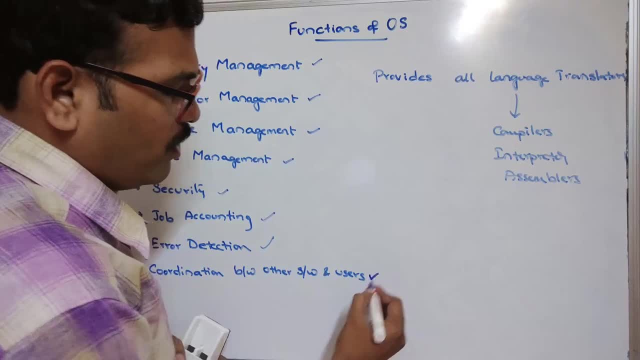 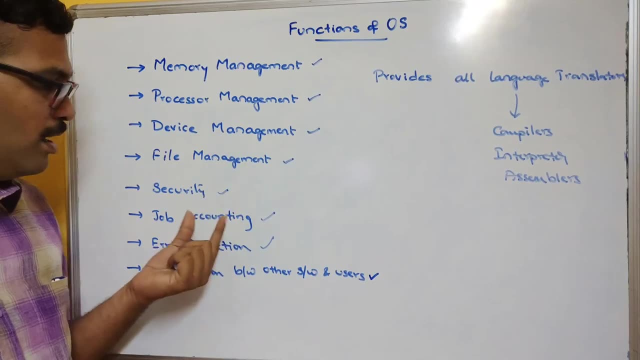 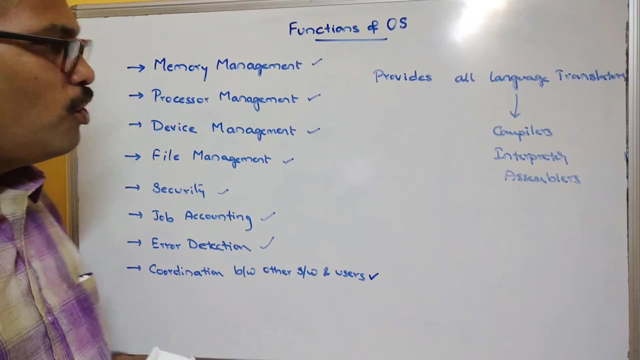 all the functionalities of, I mean the functions of operating system. so one is the memory management, processor management, device management, file management, security, job accounting, error detection and the coordination between the softwares and the users, right? so hope you understood this one and in our further concepts we'll be 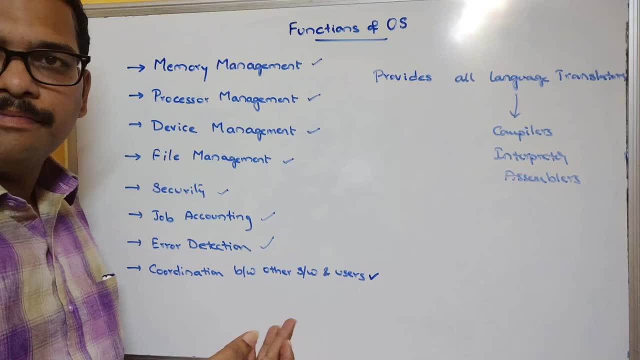 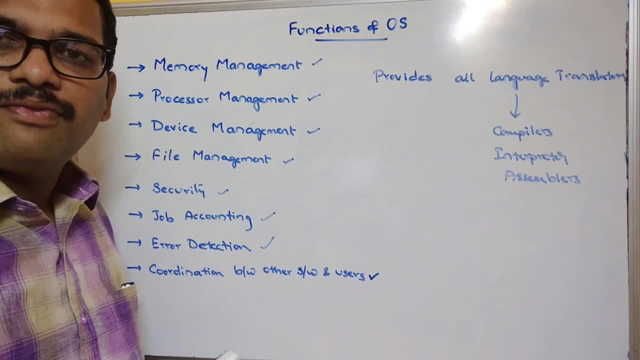 we will be discussing about all these things in detail. right, so let's stop here and hope you understood this one, and if you are having any doubts regarding this one, feel free to post your doubts in the comment section. definitely, I will try to clarify all your doubts and, if you really enjoyed my session, like my session, share my session with. 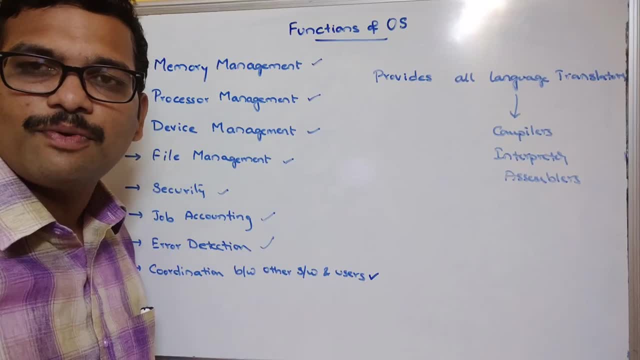 your friends and don't forget to subscribe to our channel. thanks for watching. thank you very much.